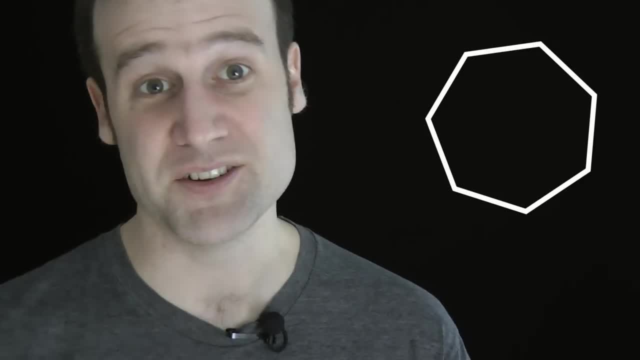 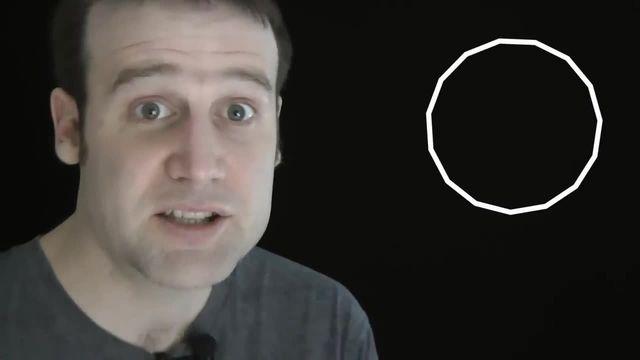 then the regular pentagon and so on. There are hexagons and heptagons, there are octagons and nonagons. It carries on for ages, gradually just looking more and more like a circle. And that's the problem in 2D: There aren't enough limitations, There are technically 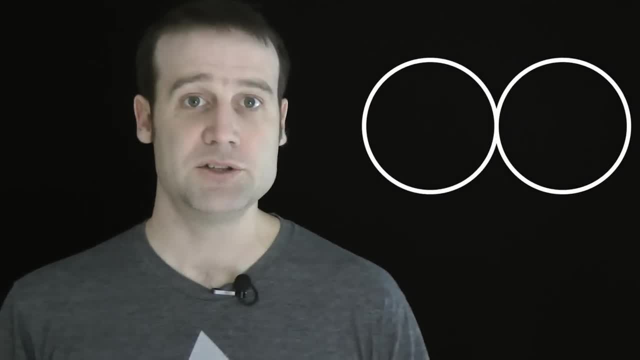 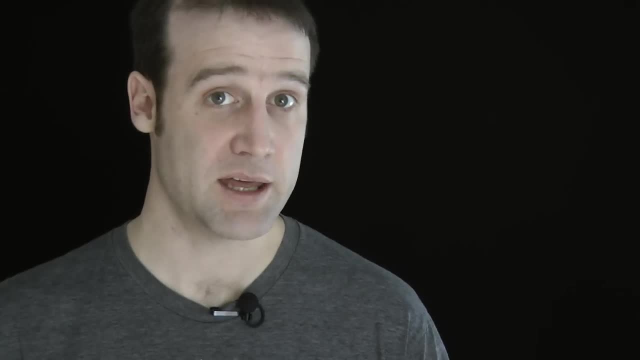 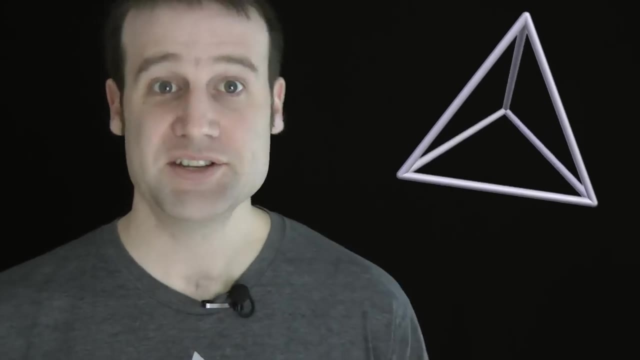 infinitely many possible regular 2D polygons. In 3D, however, things get a lot more interesting. We can join 2D polygons together to make 3D polyhedrons, Polyhedra, Whatever. More importantly, here I have one of them. This is a tetrahedron and it is a regular. 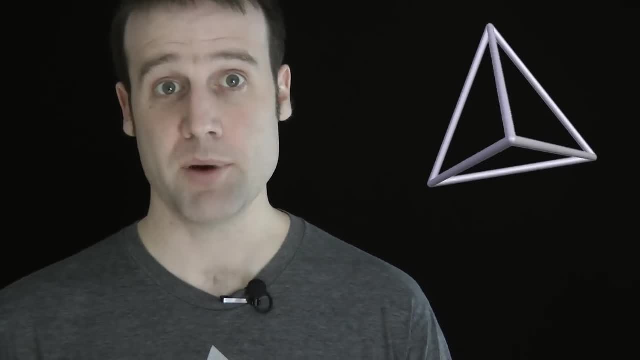 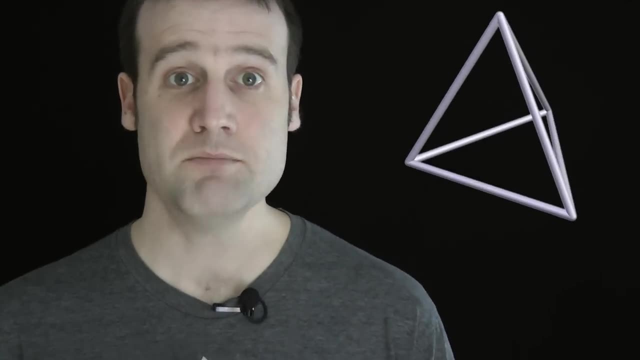 polyhedron, which means not only are its faces made up of regular polygons- in this case you can see they're all equilateral triangles- but on top of that, where those regular 2D faces meet, form identical vertices in 3D And regular polyhedrons. 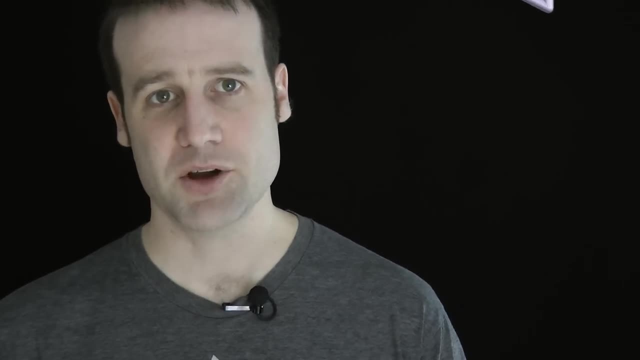 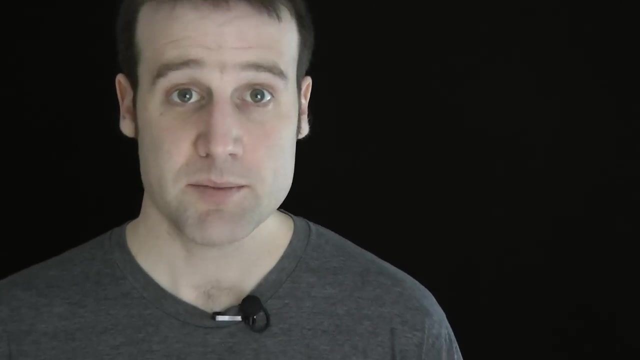 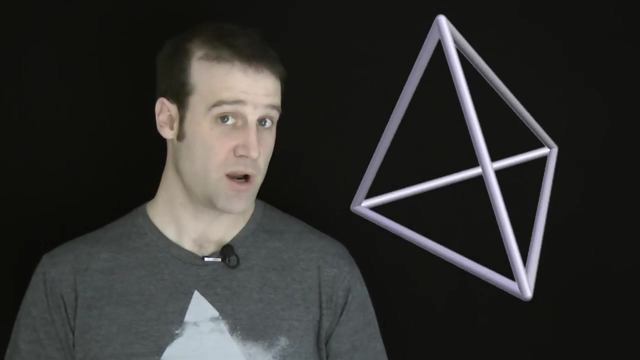 are far more exciting than regular polygons, and that's because they're a lot rarer. There are only five possible versions of this shape. We call them the platonic solids because Plato absolutely loved them, and here they all are. Number one: the tetrahedron made of four identical equilateral triangles that all meet three to a vertex. 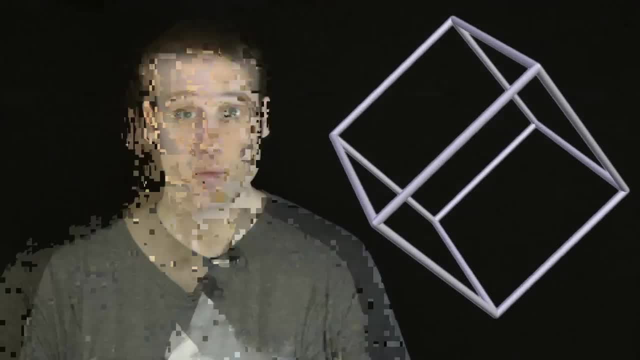 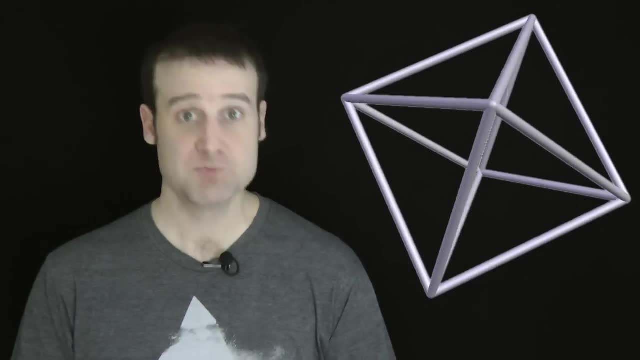 Number two, the cube made of six identical squares which, like the tetrahedron, all meet three to a vertex. Number three, the octahedron, also made of identical equilateral triangles, but this time joined four to a vertex. 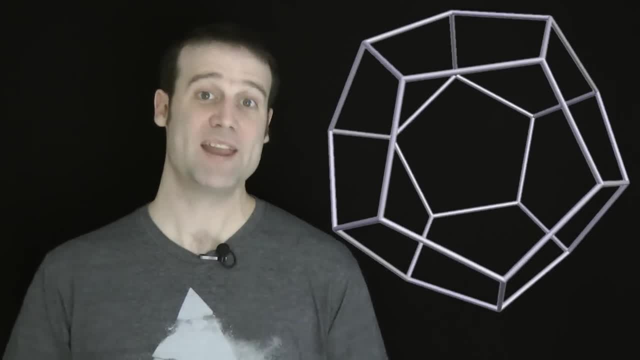 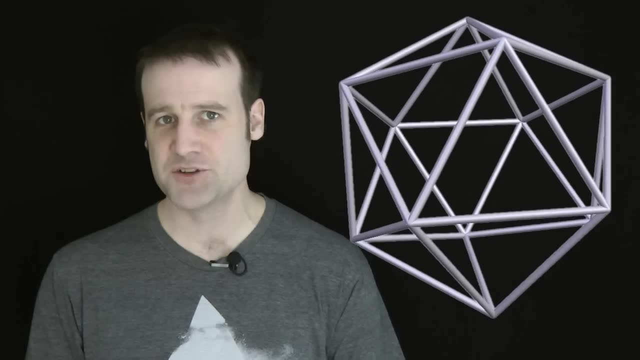 Number four, the dodecahedron, made of 12 identical regular pentagons joined three to a vertex. Number five, the icosahedron: 20 identical equilateral triangles joined five to a vertex. And then that's it, Despite the infinitely many 2D regular shapes. 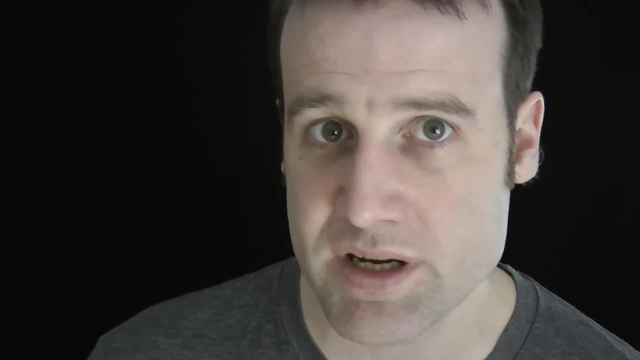 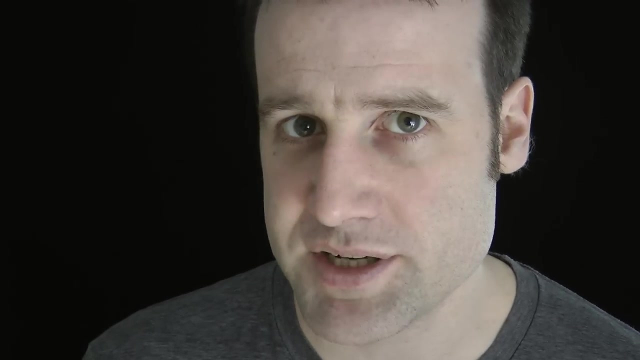 there's no other way to join them together to make a regular 3D shape. We only get those five platonic solids. Euclid even finished his series of books, The Elements, in Book 13,, Proposition 18, with the proof that there are only five of them. 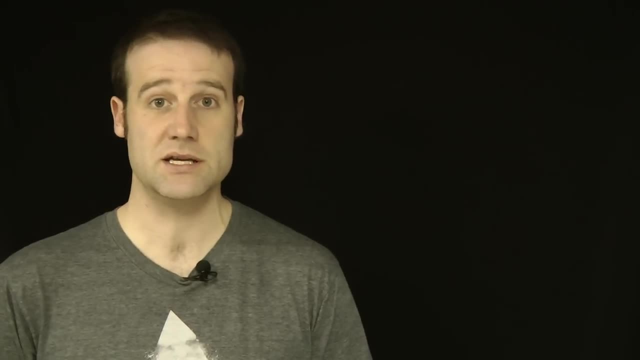 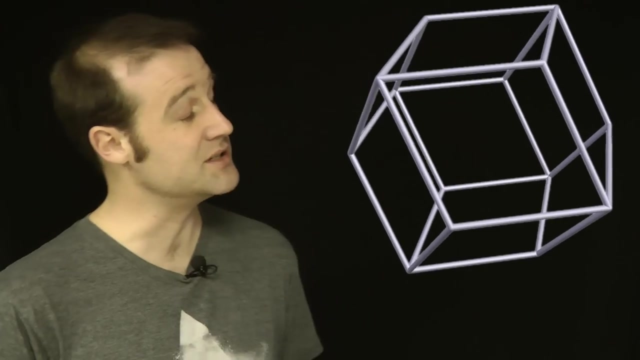 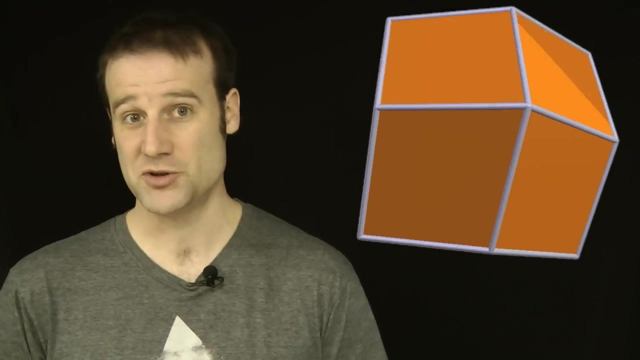 Which is not to say there aren't some other great 3D solids. This here is a rhombic dodecahedron, Very sadly not a platonic solid, though, As you can see, the faces are diamonds. Diamonds where, if they were one high, they're exactly root two across. 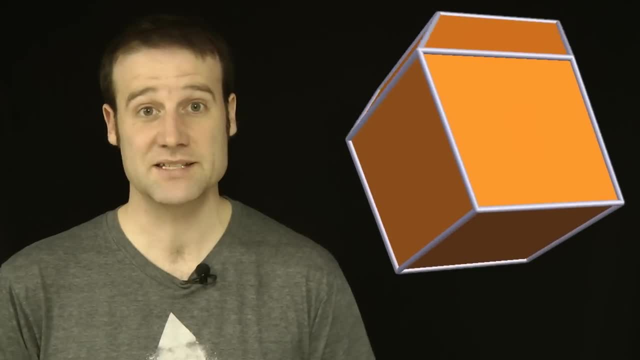 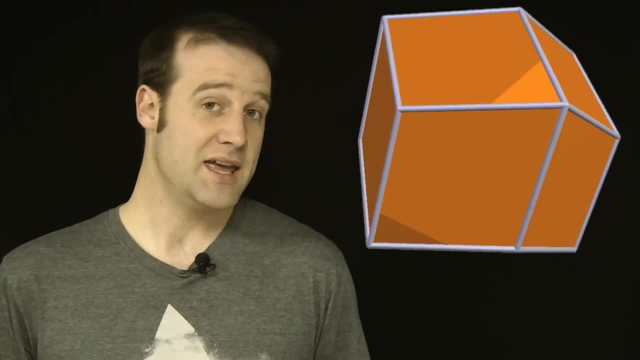 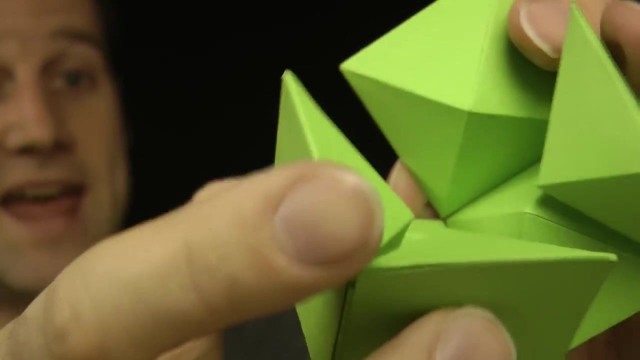 And all the vertices aren't the same, but still fantastic shape And it does link to one of the platonic solids. You see, the rhombic dodecahedron is a cube turned inside out. Here I have a model of a solid cube, but made from a net of triangular pyramids. 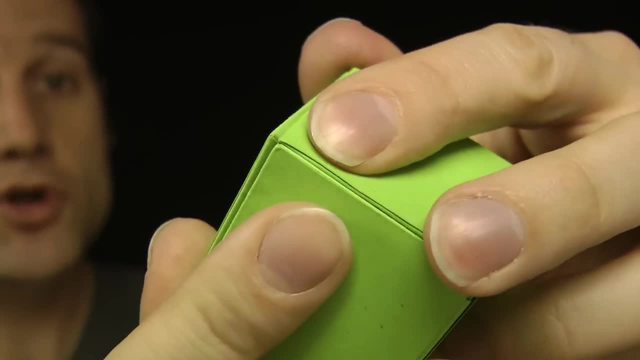 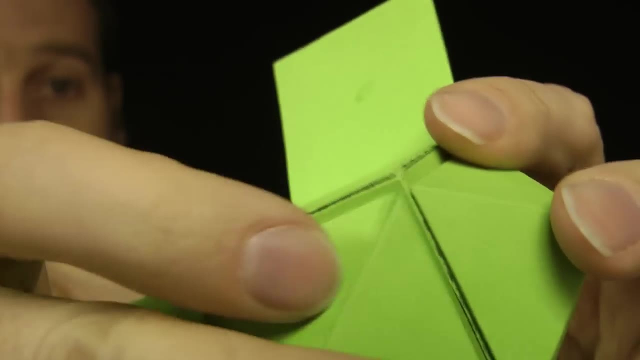 So if you put it back together this way, you get the original solid cube. If you put it back together inside out, though- and this helps- if you put a solid cube in the middle to hold everything in place- the shape you end up with. 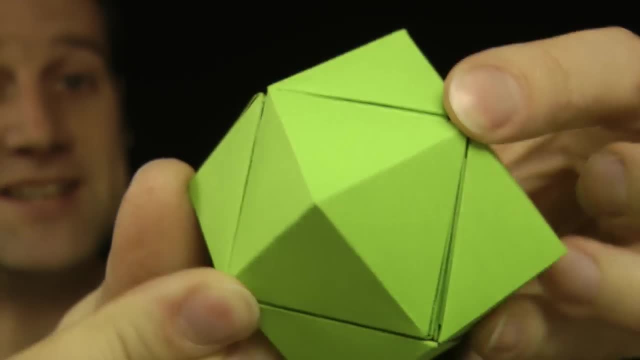 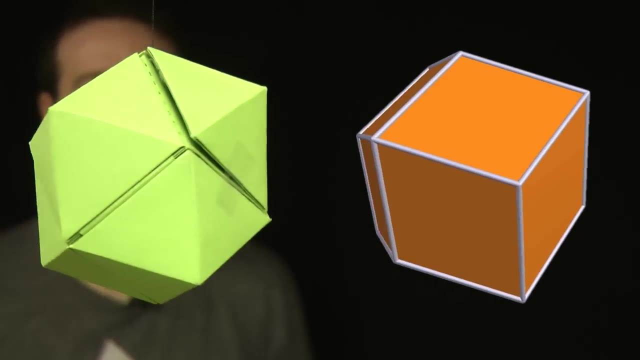 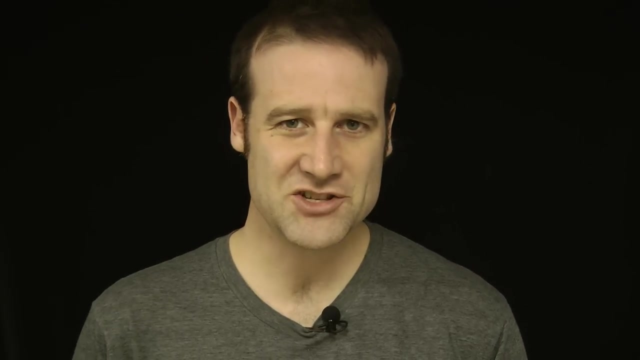 is a rhombic dodecahedron. So an inside-out cube is a rhombic dodecahedron. Hang on, hang on. Yes, Look at that. Eh, Eh. It carries on into the fourth dimension. 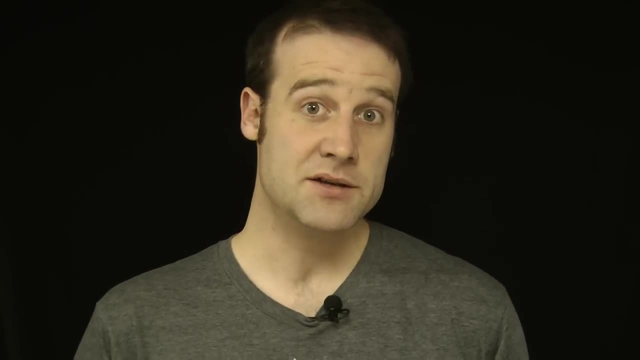 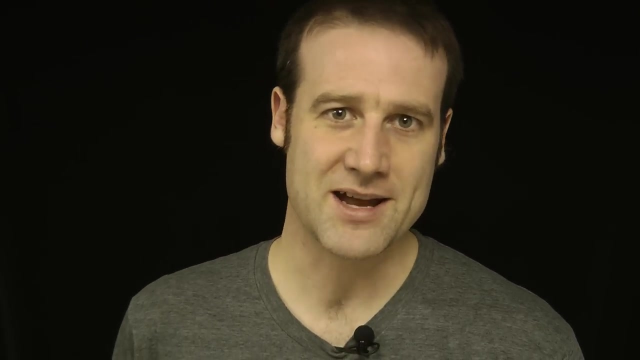 Just like you can join regular 2D polygons together to make a regular 3D polyhedron, you can then join regular 3D polyhedrons together to make a regular 4D polychoron, And all five of them are here. 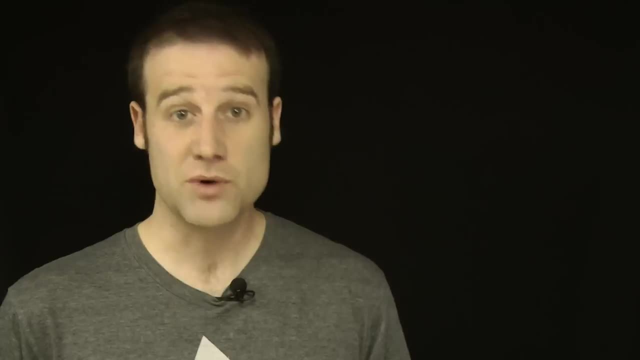 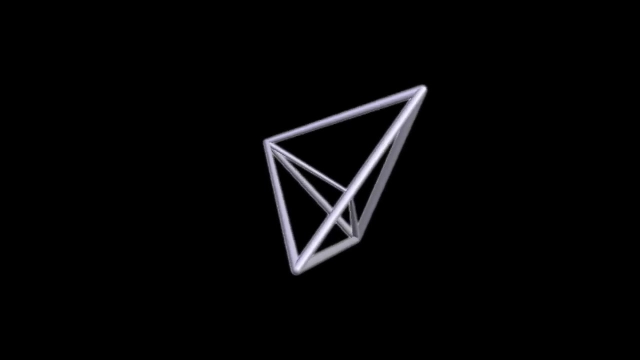 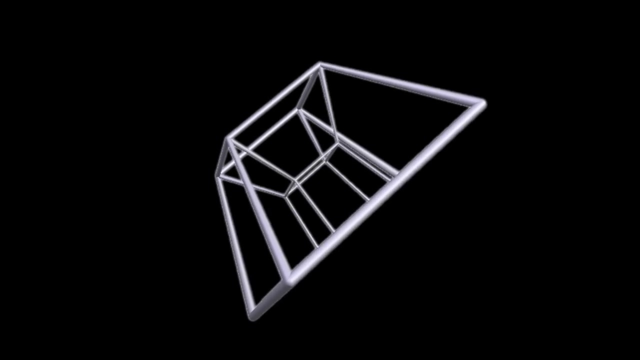 If you join regular tetrahedrons together, three to an edge, five of them together in the fourth dimension will make the hyper-tetrahedron. Eight cubes joined three to an edge will make for a hyper-cube. Sixteen tetrahedrons joined four to an edge give the hyper-octahedron. 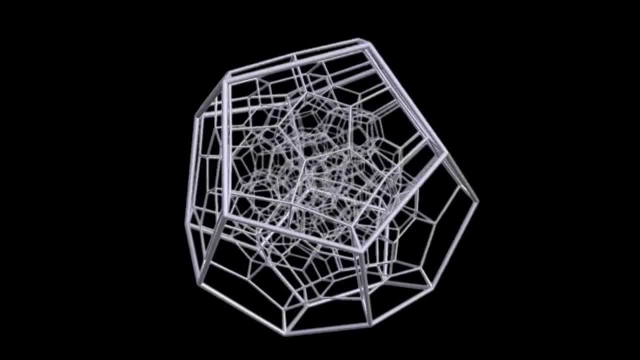 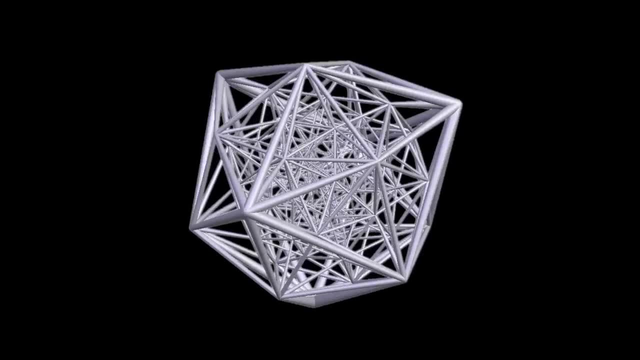 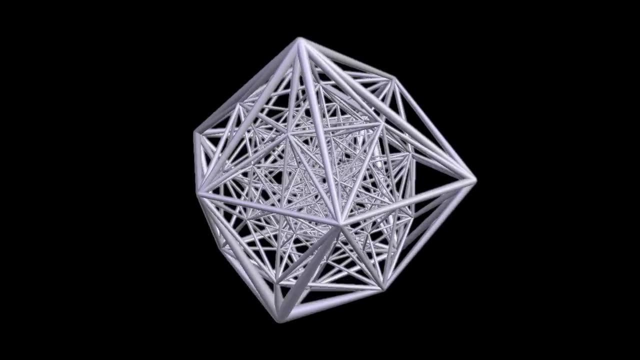 A hundred and twenty regular dodecahedrons all join three to an edge to make the hyper-dodecahedron. And finally, if you have six hundred tetrahedrons lying around, you can join them five to an edge to make the hyper-icosahedron. So there you have it. In 4D, you still have five platonic solids, except suddenly there's one more. There's a sixth platonic solid, There's a seventh platonic solid in 4D, and it's the 4D equivalent of the rhombic dodecahedron. 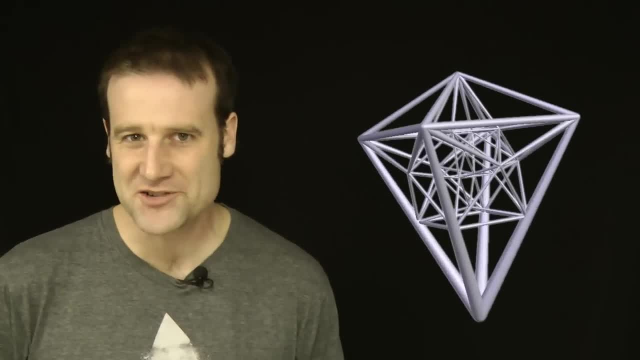 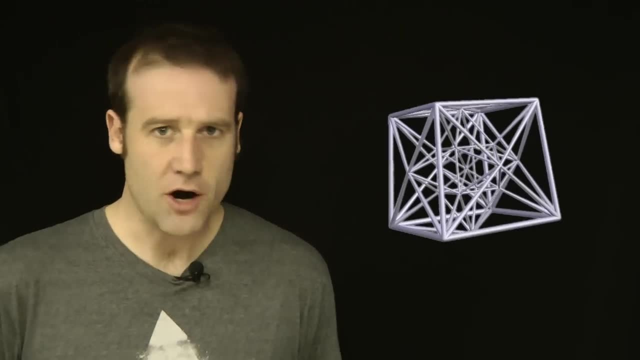 Check it out. That is 24 octahedrons all joined together three to an edge, and in 4D it is a platonic solid often called the icosahedron or the octa-cube. I prefer it by its name: the hyper-diamond.